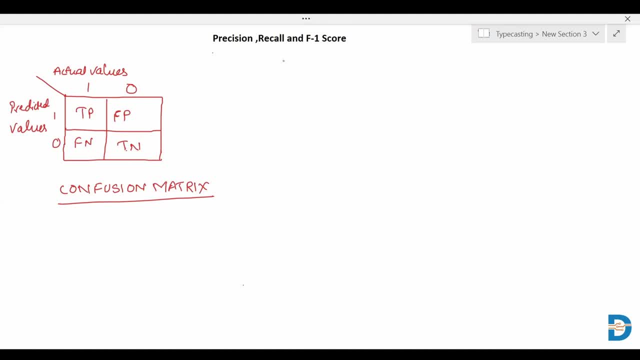 so now, what is precision? recall and f1 score, these are the evaluation, or you can say performance matrices extracted from the confusion. matrix for classification model: okay, for classification models. okay, these are the evaluation performances, evaluation parameters, okay. so let's understand first what is precision? precision is out of total predicted. 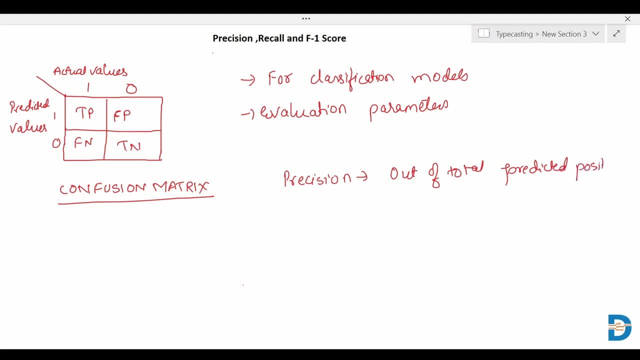 out of total predicted positive result, how many results were actually positive? how many results were actually positive? okay, so the formula for precision is given by tp divided. So out of total predicted positive values, how many are actually positive? Okay, What is recall Recall? 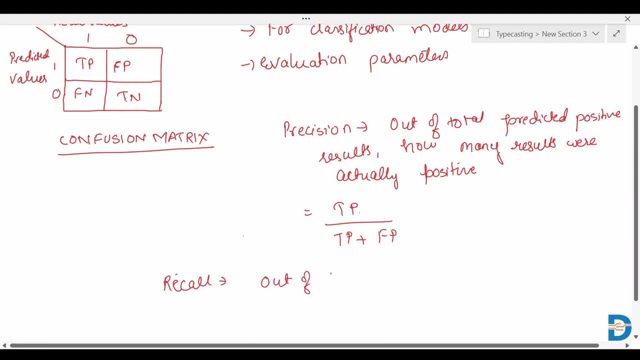 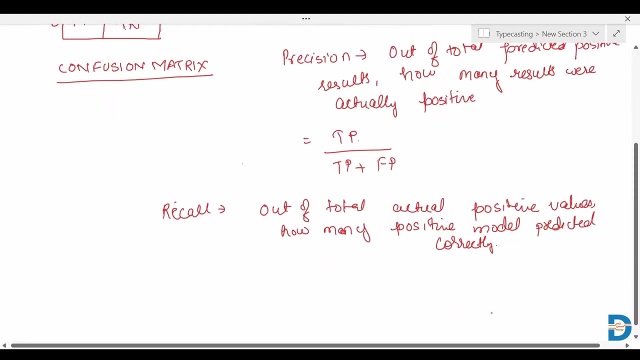 Recall is given by: out of total actual positive values, Recall is how many positive model predicted correctly. Okay, So the formula for recall is TP, that is true positive divided by true positive plus positive, False negative. So out of total actual positive values, how many your model predicted correctly? 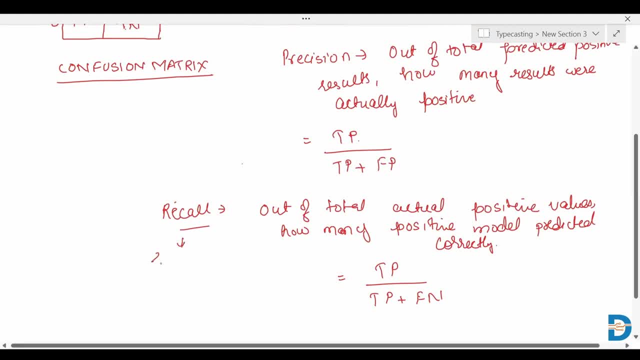 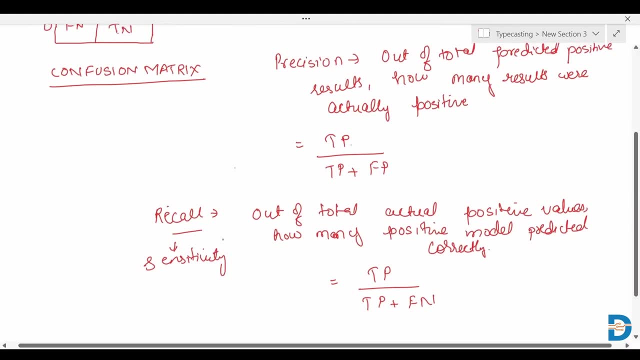 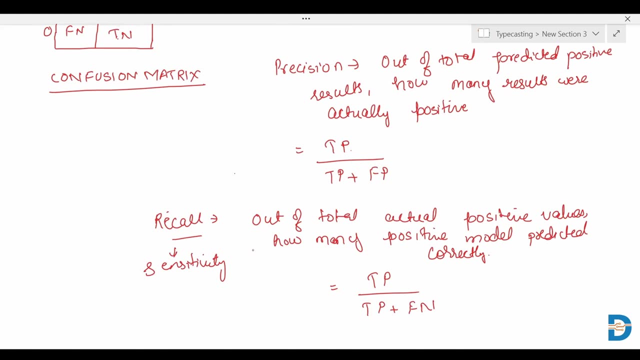 This is given by recall. Recall is also known as sensitivity. Okay, So in some of the data set, precision is important. In some of the data sets, recall is important. Okay, But when both are important, we'll come towards.